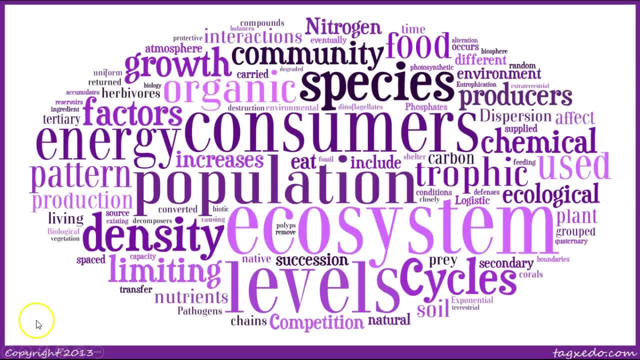 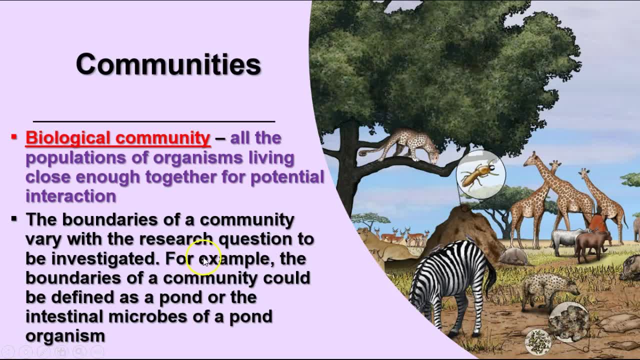 In ecosystems. populations don't live by themselves. They actually interact with other populations and that's called a community. A community is all of the populations of organisms living close enough together for interaction in a particular environment. The boundaries of the community can depend on what you're talking about. 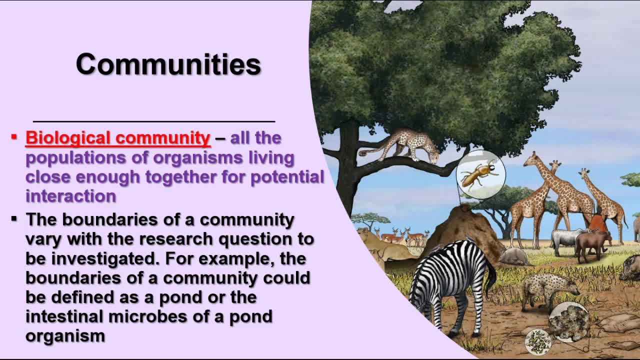 If you're just talking about all the different animals and plants that live in your backyard, then that would be the limits of the community for that particular study. You could also have a pond. You could also talk about the microbes that live in the intestines of a fish, that live in the pond. 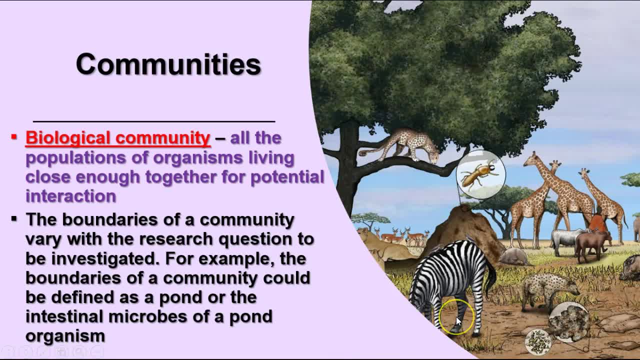 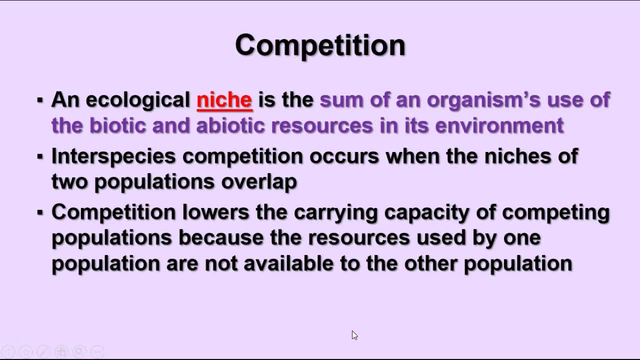 There are lots of different ways to define a community, but basically you have all the different organisms that live and interact with each other in that particular environment. When we talk about communities, we also have to talk about various ways that the organisms interact with each other. 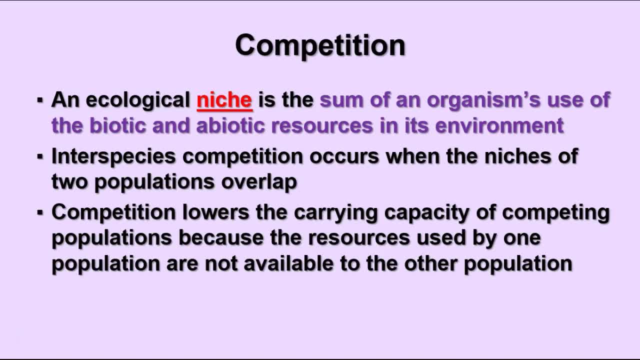 One way that we do that is to talk about the ways that they compete with each other. An organism's use of the biotic and abiotic resources of its environment is called its niche. This is basically like the occupation of the organism within its habitat. 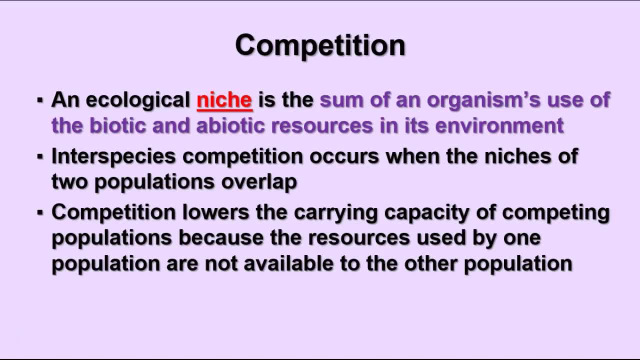 A habitat is like the address where the organism lives, and the niche is what it does within that habitat. When you end up with competition, that's when you have the niches of two different organisms, There are two different populations that overlap with each other. 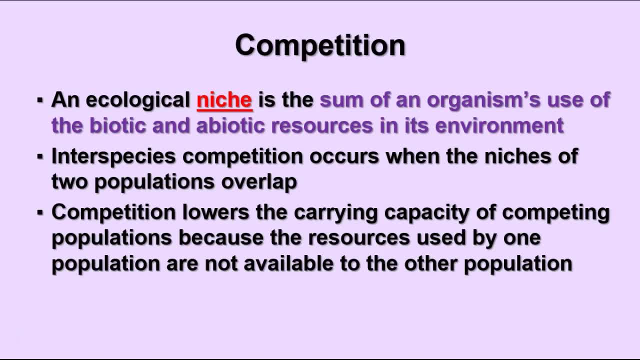 and that can lead to various kinds of competition. They can work together, they can work against each other, all different kinds of things like that. One thing to keep in mind when you think about this in terms of populations is that competition is going to lower the carrying capacity of both of those populations. 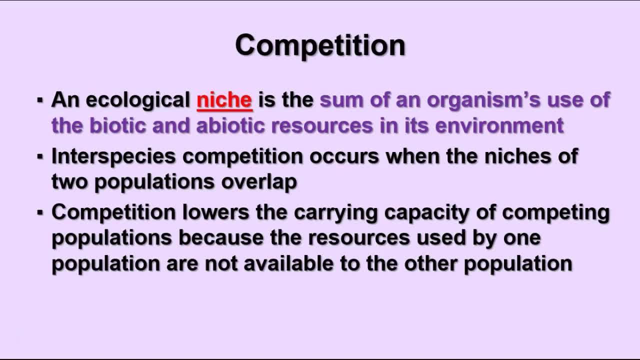 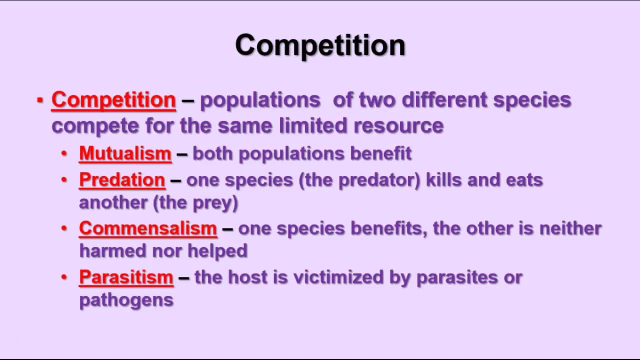 because the resources can't be available to both populations at the same time. There are various kinds of competitions that can occur within environments. One type is mutualism. In mutualism, both populations benefit from the relationship with each other. They both get something out of the relationship. 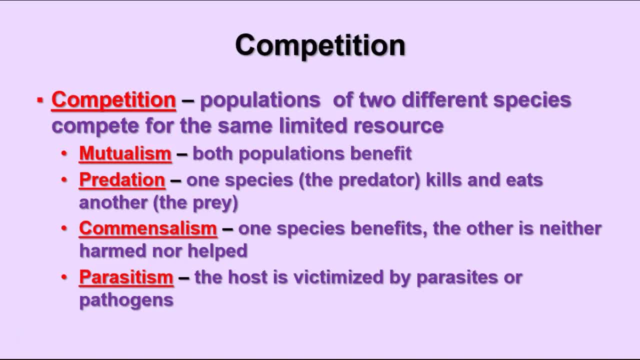 In predation you've got one species that kills and eats another. That's the predator, kills and eats the prey. Commensalism is when you have one species that gets some benefit from the relationship. the other is neither harmed nor helped. 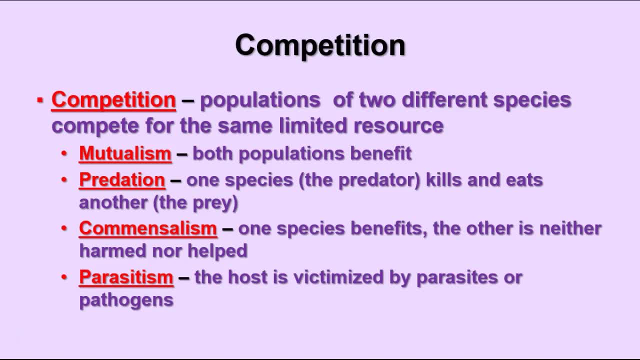 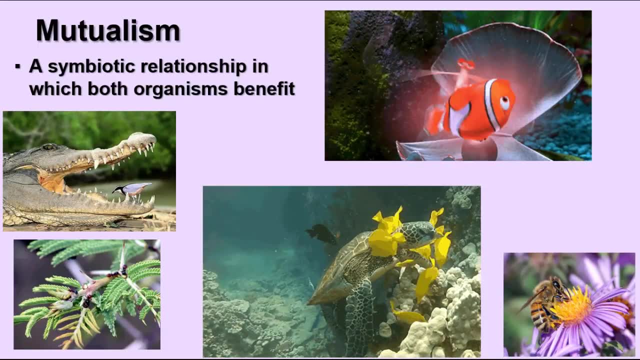 And then the fourth kind is parasitism, and that's when you have a host that is victimized by parasites or pathogens. So let's look at some examples of all those kinds of things In mutualism, when you have both species benefit from something. 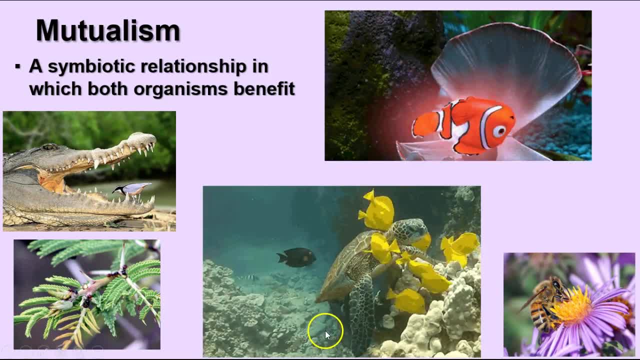 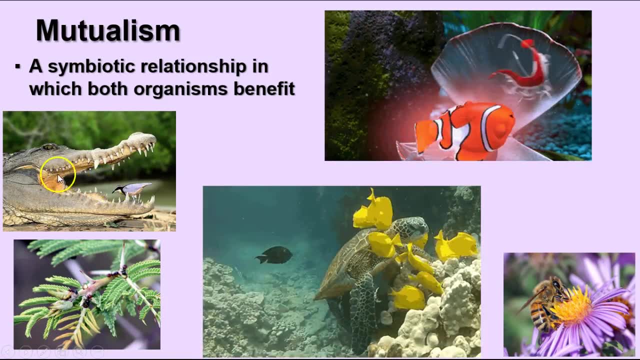 here we see several different examples of mutualism. Of course, a cute example up here from Finding Nemo, but we've also got this bird that actually picks the teeth of the crocodile, and the crocodile benefits because it gets all the stuff out of its teeth. 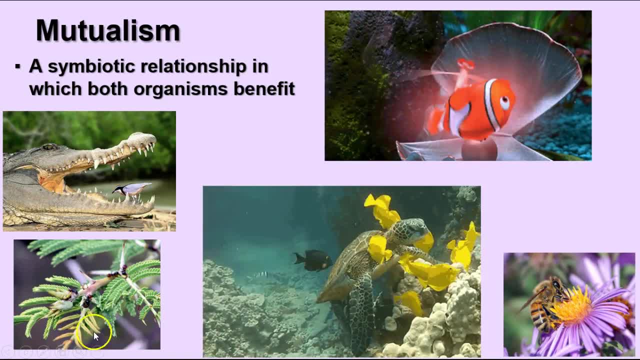 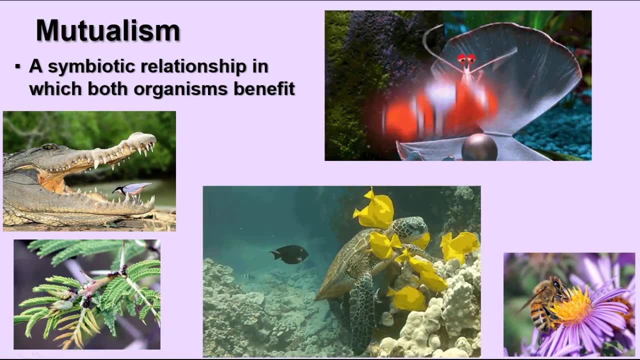 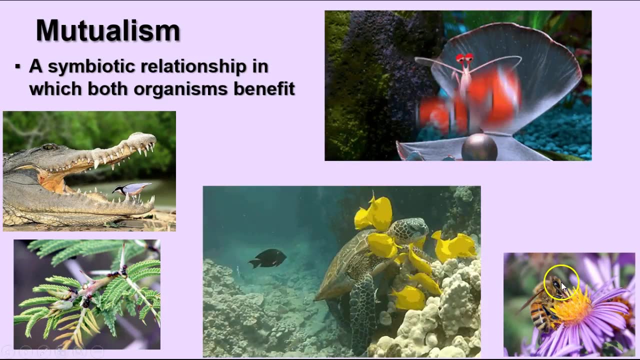 and the bird benefits because it gets something to eat. This tree down here is inhabited by ants that actually help protect the tree from other invaders, and the tree provides the food for the ants And even bees and flowers. The bee gets the benefit of getting the pollen and getting the nectar to make the honey. 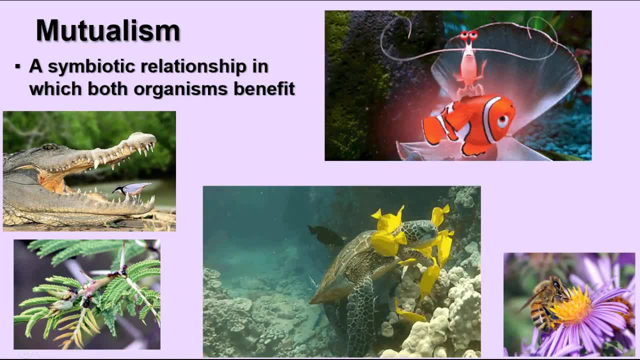 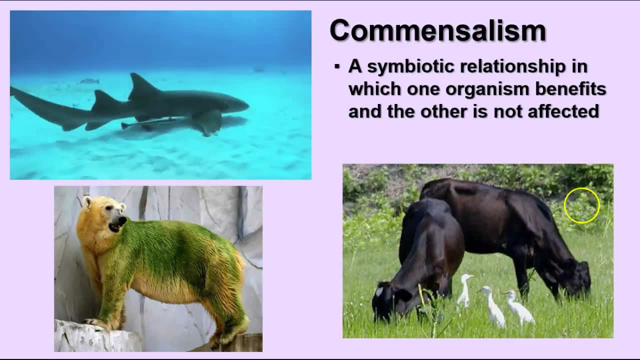 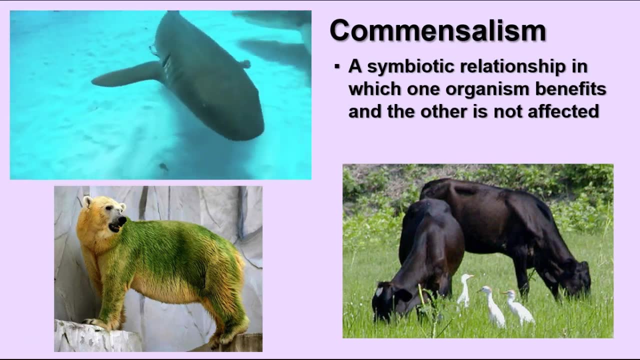 but it also pollinates flowers, which provides for some variety in the gene pool of the flower species. Another relationship is commensalism. This is when you have one organism that gets some benefit from the relationship and the other one is not really affected one way or the other. 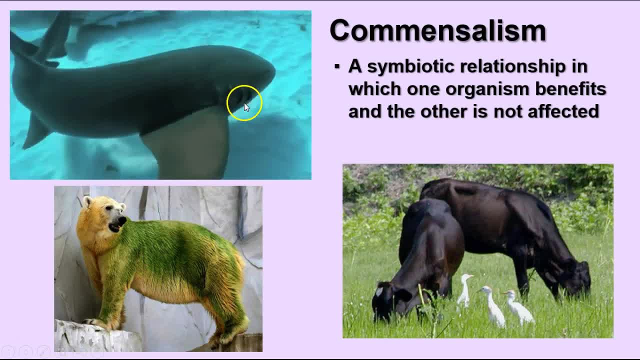 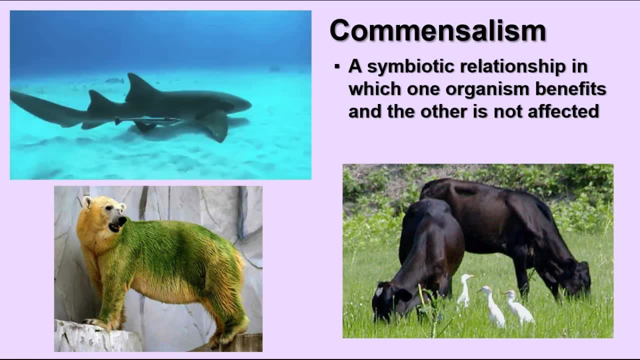 We see several examples here. At the top left we've got a shark with a remora. A remora is a fish that kind of hangs around with a shark and basically the remora can hitch a ride onto the shark and go from place to place and also eat the shark's leftovers. 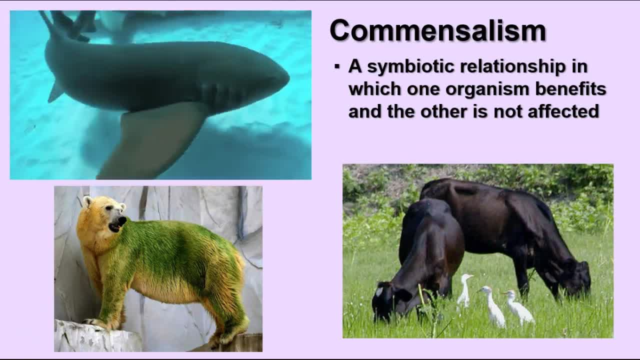 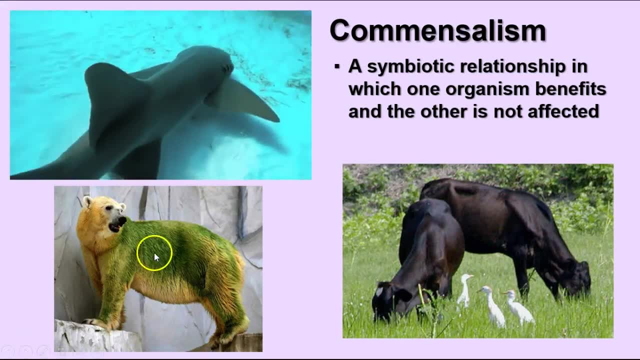 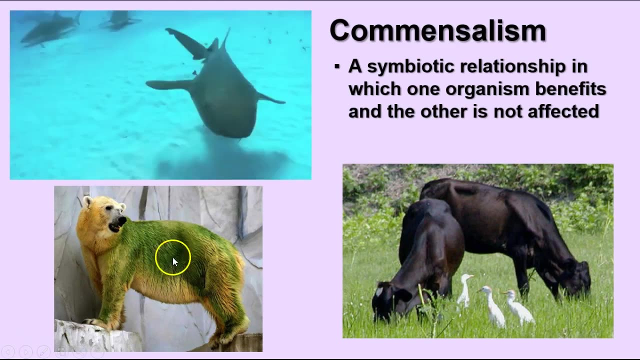 The shark isn't bothered one way or the other with the remora. It doesn't eat the remora, it isn't bothered by it and it doesn't really help it at all. You might wonder about this relationship. This is a polar bear that's got algae growing on it. 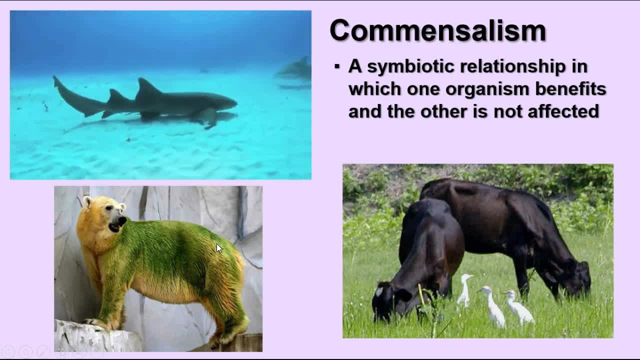 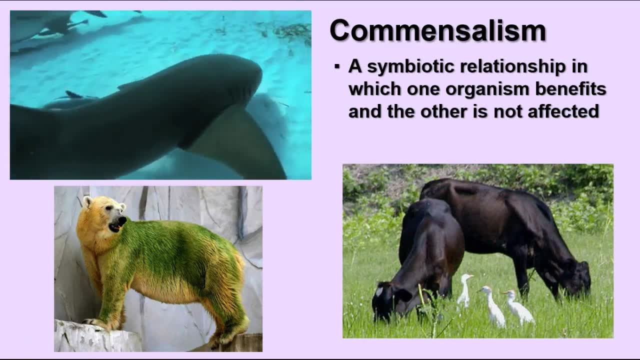 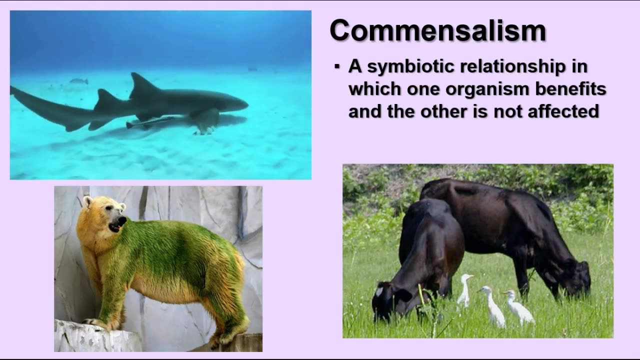 Now, polar bears have hairs that are hollow, and that's one of their adaptations that allows them to live in the cold climates that they live in, But when they live in warmer places, these hollow hairs on their fur actually provides a place for algae to live. 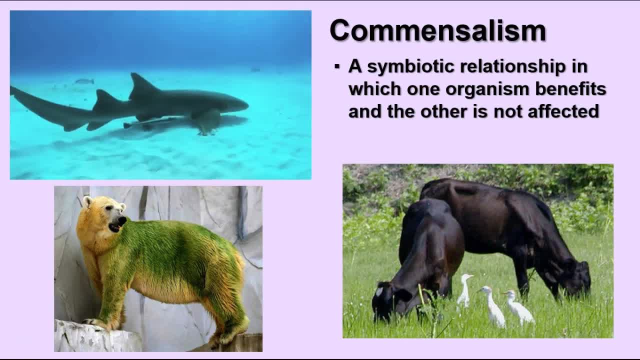 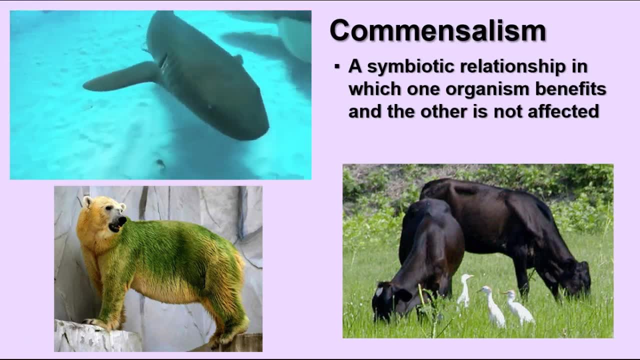 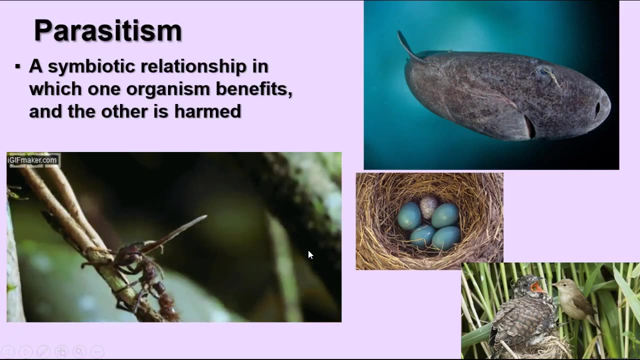 The algae gets the benefit of having the warmth and the water from the polar bear, but the polar bear's not either bothered nor helped by the algae being there. Another example would be parasitism. In parasitism you've got one organism that benefits. 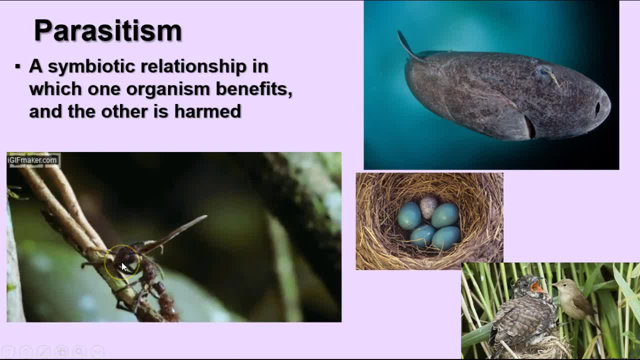 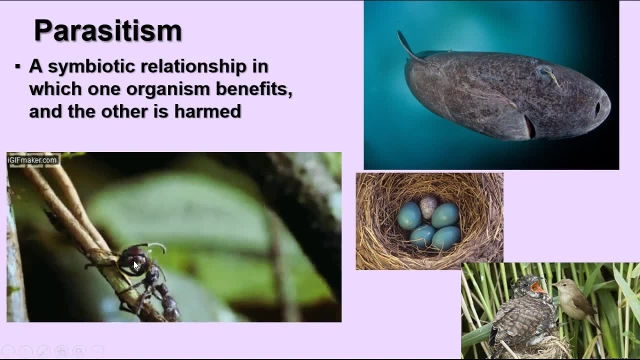 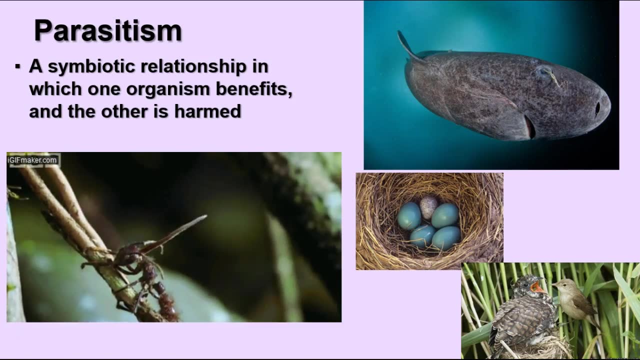 and the other one is harmed On the lower left. we see an example here of a type of fungus called a cordyceps fungus that actually attacks various kinds of insects and actually eats its way through their bodies and eventually kills it. The insect's body provides food for the fungus to grow and reproduce. 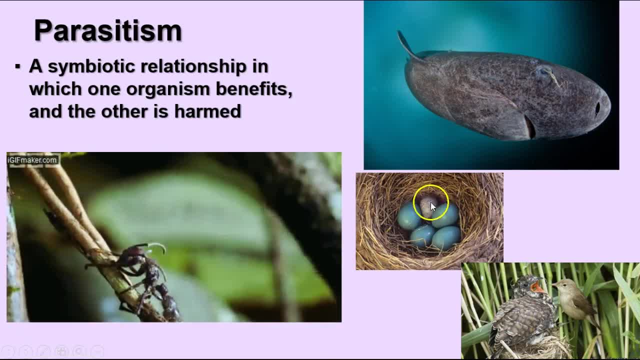 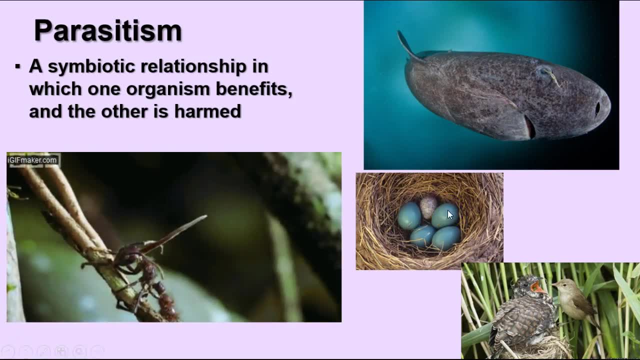 Here we have a clutch of eggs, with an extra egg of a different species in there, probably something like a cuckoo. Cuckoos oftentimes will lay their eggs in another bird's nest and let the other bird hatch its own young and feed it. 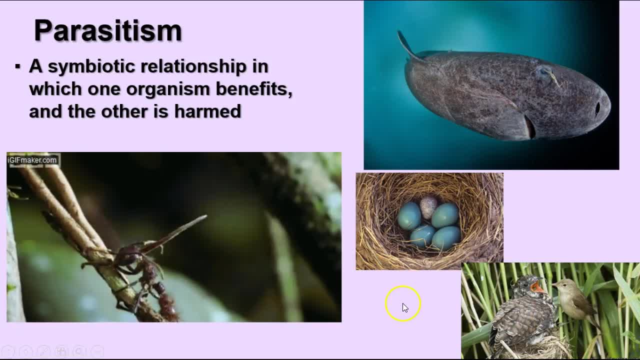 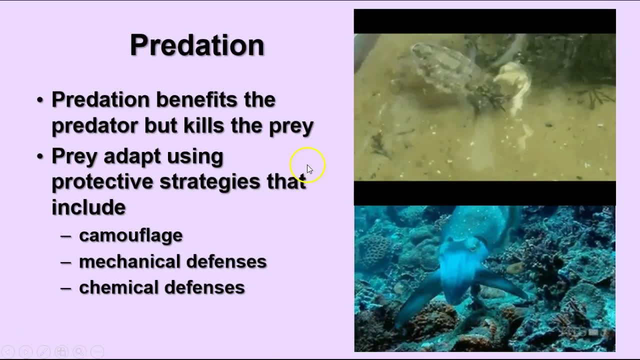 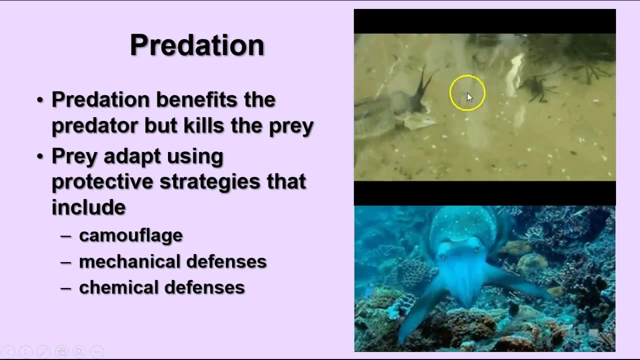 So there are lots of examples of parasitism in nature. In predation you've got a benefit for the predator but the prey gets killed in the process. Here we have a type of snail- This is a cuttlefish- and the cuttlefish is catching a little crab here and eating that. 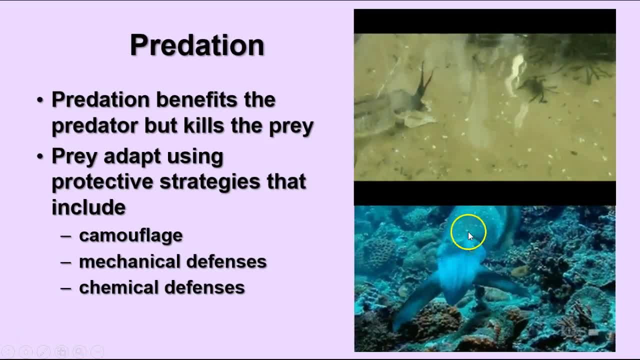 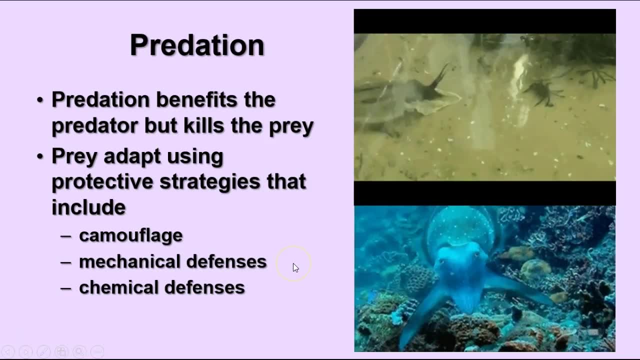 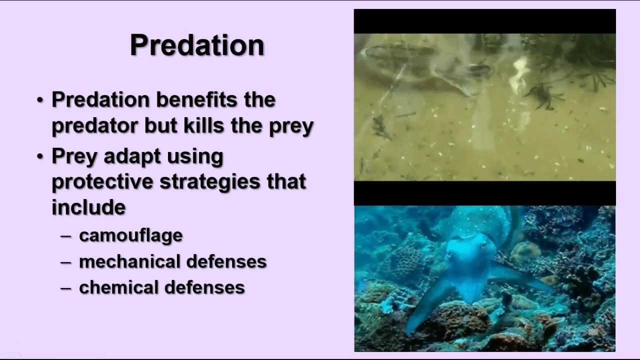 This shows the way the cuttlefish actually mesmerizes or kind of hypnotizes its prey. And prey have to adapt to protective structures of some kind or another. One of the very common things that they do is develop some kind of camouflage. They also have various mechanical defenses and chemical defenses. 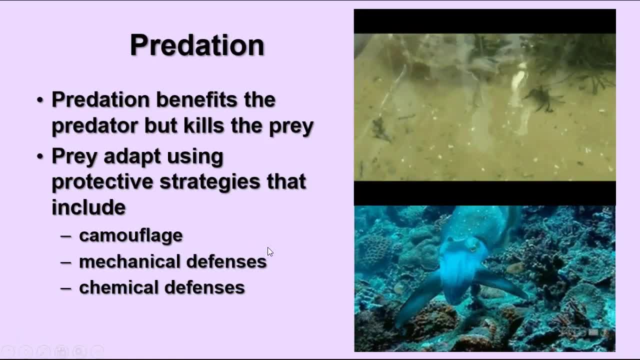 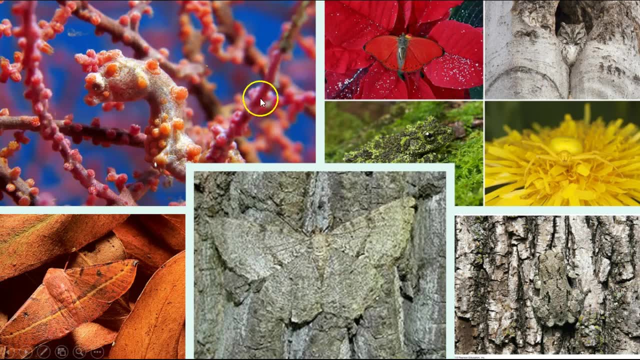 that can help protect them from the predators. Here we have a seahorse. The seahorse has a way of hiding. This is in a coral reef and there are actually little protuberances on the surface of the seahorse that look like the coral polyps growing out of the coral. 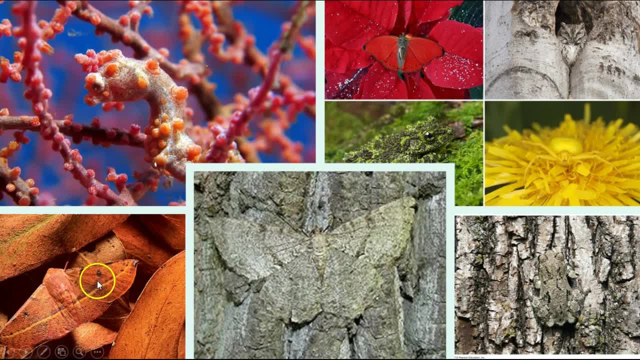 We have various examples with insects. Here's a type of moth that looks very much like leaves. Here's another moth that can blend in with the tree. Another moth that looks like a flower there, And then other kinds of insects. Here's an insect that's hiding. 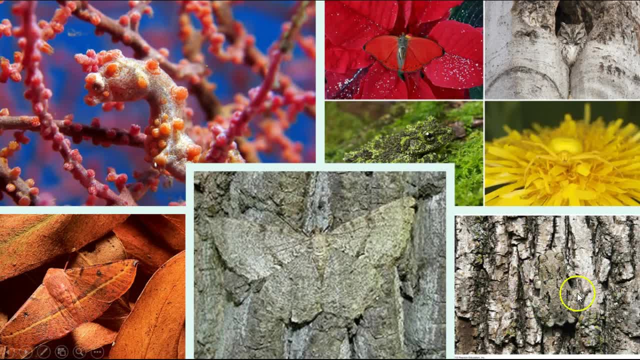 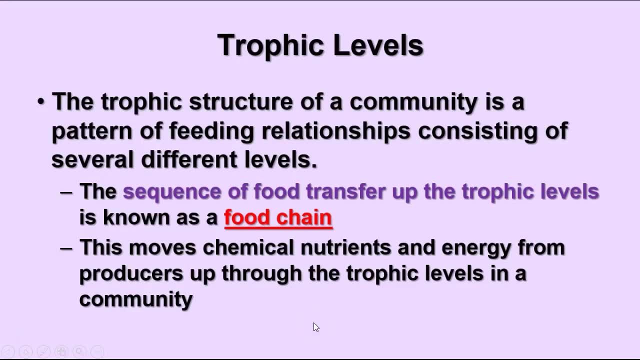 Here's the same coloration as the flower it lives on. Here's a frog that blends into the tree there. So there are lots of examples of those kinds of things in nature. Now, when we talk about those relationships within a community, we have to talk about the feeding relationships. 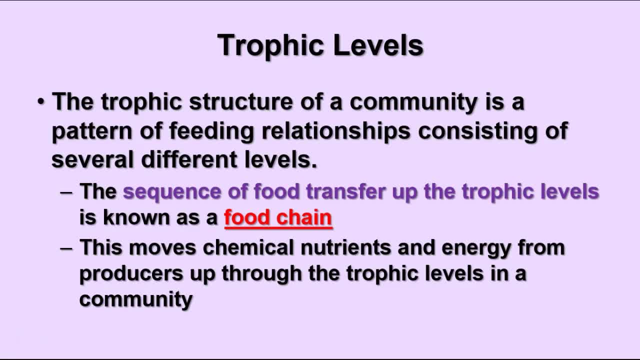 and these are called trophic levels. If you think about it, trophic just means feeding, And so when we look at the sequence of the food transfer up the trophic levels, we call that a food chain, And what this does is it recycles. 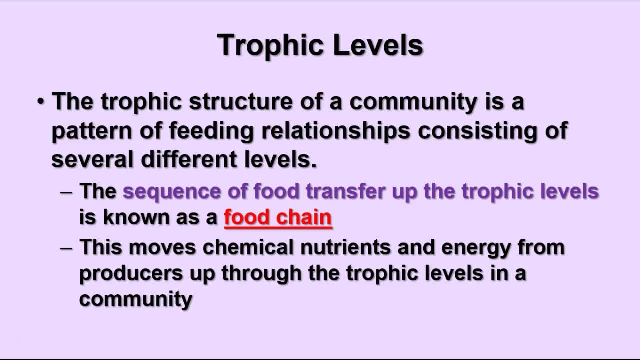 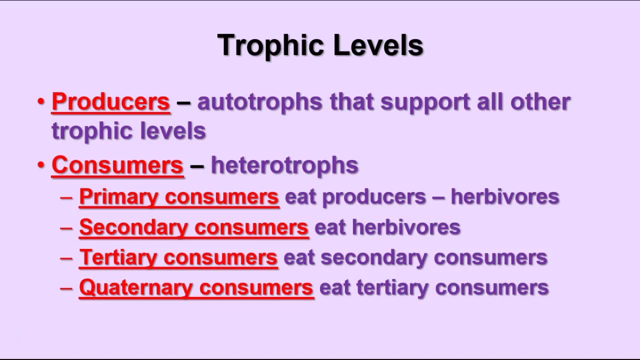 and moves the chemical nutrients and energy through the trophic levels in a community from the producers to the primary and secondary and tertiary consumers. So the producers are autotrophs like plants that support all the other trophic levels. Plants generally are the main source of food in terrestrial ecosystems. 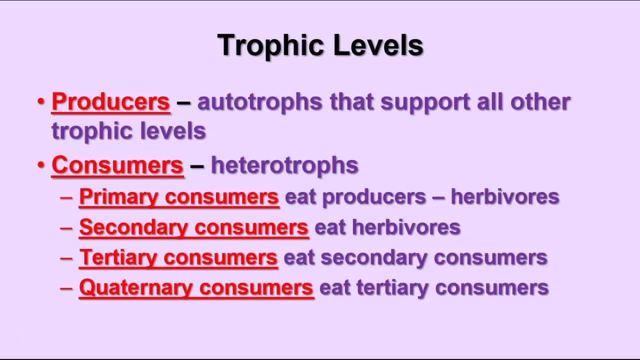 In aquatic ones it would be something like algae, But those are still a photosynthetic or an autotrophic organism that's going to provide the basis of the food chain. The consumers are the heterotrophs of various kinds, And so we have primary consumers. 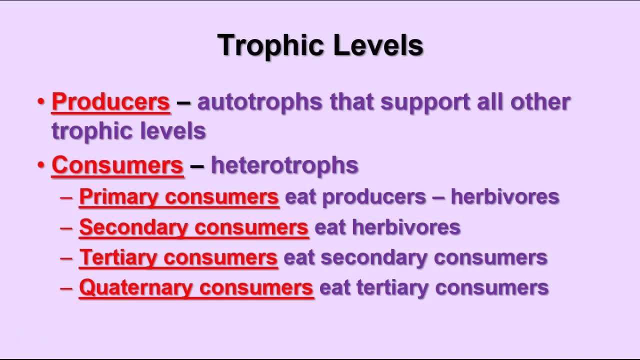 those are the organisms that eat the producers. those are herbivores. We have secondary consumers that eat the herbivores, Tertiary consumers eat the secondary consumers and quaternary consumers eat the tertiary consumers And we think about that. it makes a very nice little chain. 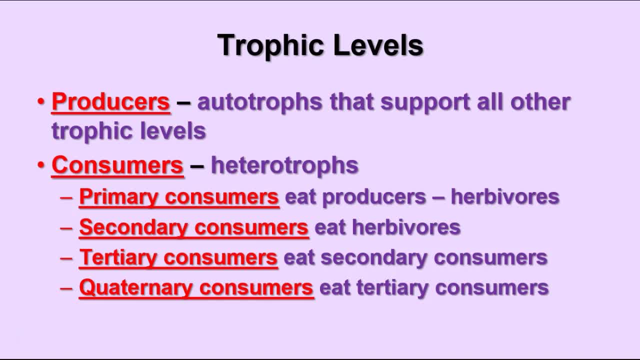 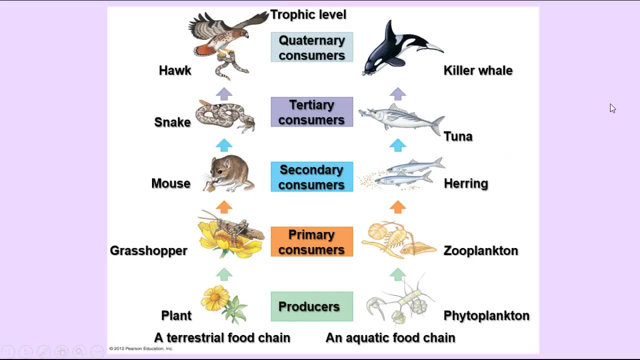 However, within that chain, most organisms don't eat just one thing. They actually it depends on. they're classified at different levels: primary, secondary and so forth, depending on that particular thing that they've just eaten. Okay, Here we have a couple of examples of food chains. 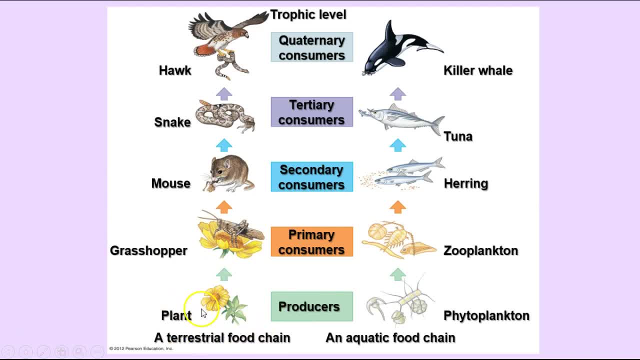 A terrestrial food chain over here would begin with the plant And then the primary consumer of the plant in this case is a grasshopper. When the mouse eats the grasshopper, that eats the plant, that makes the mouse a secondary consumer. When the snake eats the mouse. 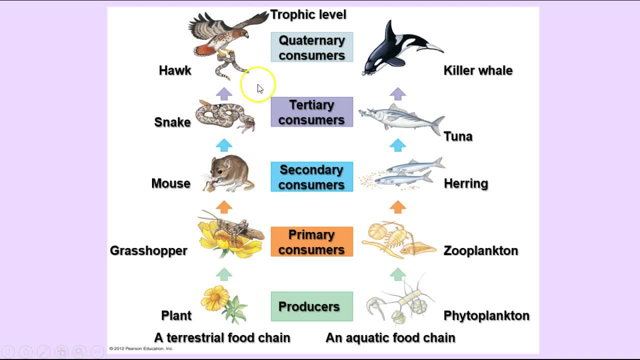 that ate the grasshopper, that ate the flower. that makes the snake a tertiary consumer, And then the hawk would eat the snake and that would make the hawk a quaternary consumer. that's the top level consumer. That doesn't mean that it eats everything else there. 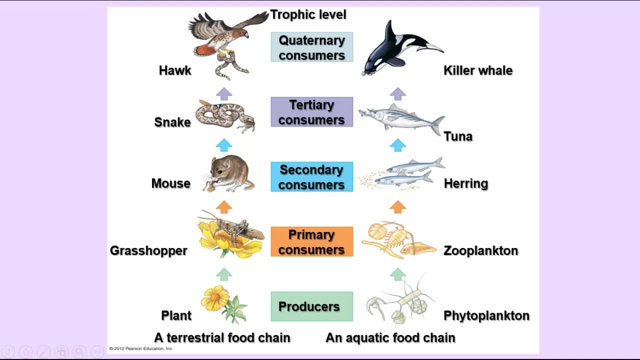 it just means when it eats that particular animal. it's at that level. In an aquatic food chain you have phytoplankton and algae. that would be the producers in that food chain. The zooplankton, the animal-like protista. 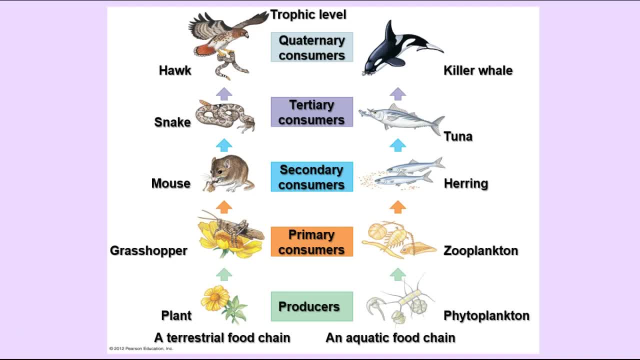 that would eat the phytoplankton. that would be the primary consumers. The smaller fish like herring that eat the zooplankton would be secondary consumers. The tuna which eat the herring would be a tertiary and the killer whale that eats the tuna. 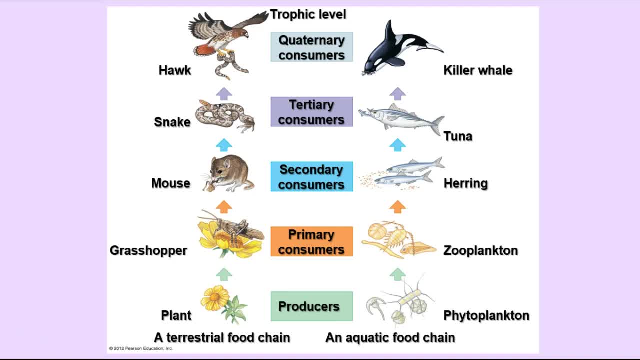 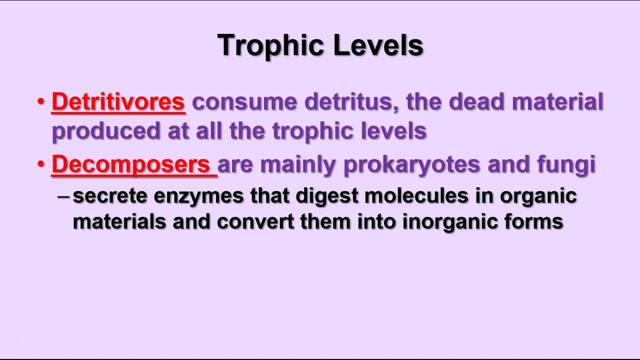 would be quaternary. We can be classified at different levels depending on what particular source of our food happens to be at that time. Now there also are other organisms that are parts of these chains. They have feeding relationships that actually don't necessarily eat. 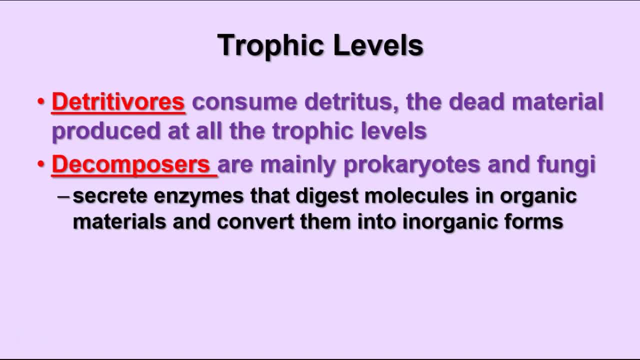 those particular things, and those are the detritivores and the decomposers. The detritivores eat the dead material that's produced at all trophic levels, the crumbs on the table, basically the leftovers. The detritivores are the things. 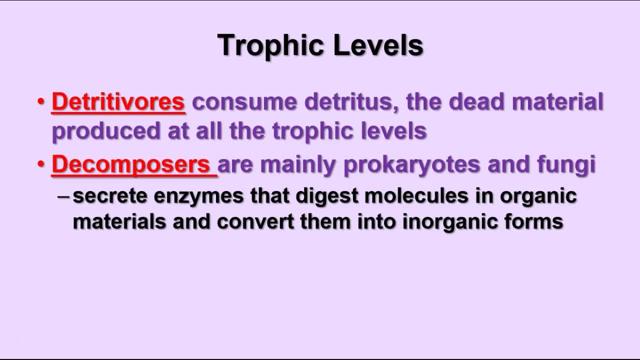 that tuna eat what's left over. Decomposers are mainly prokaryotes and fungi, and they're going to actually digest molecules in those organic molecules and those organic materials and convert them into inorganic forms that can be used by them, And those are very important. 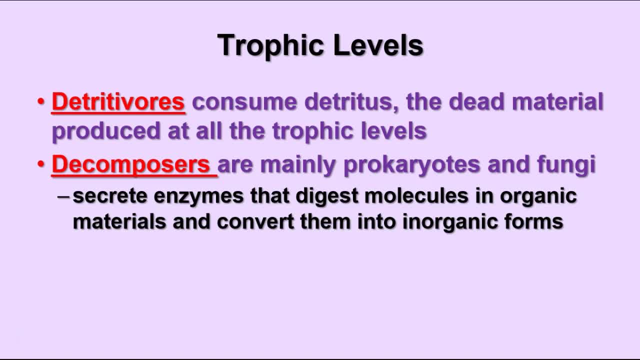 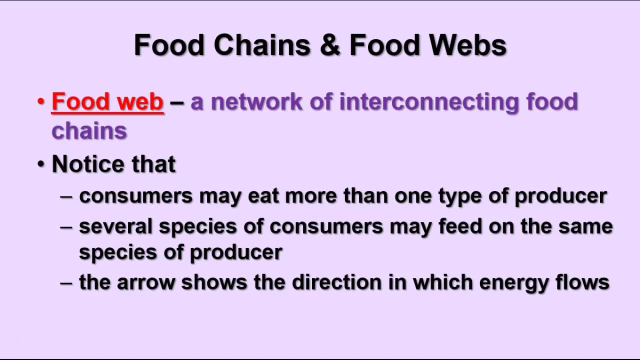 in making sure that we recycle all of the energy and all the matter within the ecosystem. A food web is the network of all the interconnecting food chains because, remember, consumers can eat more than one type of producer and then you've got several different consumers. 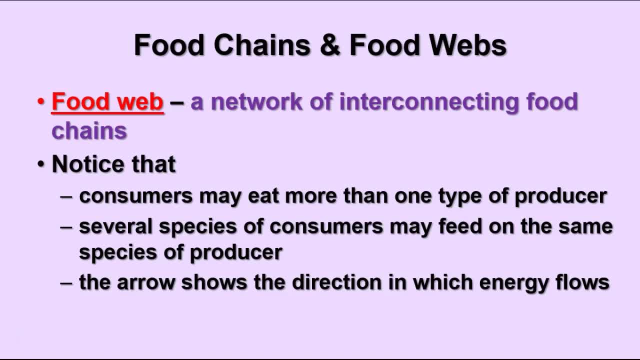 that feed on the same species of producer, not necessarily at the same time or in the same way, And so when we look at food chains and food webs- food webs in particular- the arrow shows the direction the energy is flowing: from the producer to the consumer. 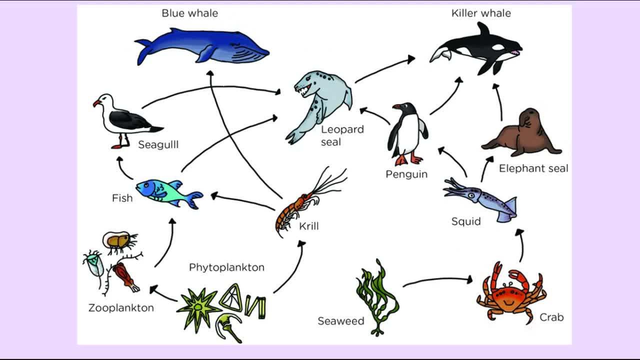 and from the primary consumer to the secondary consumer and so forth. This particular diagram shows a series of feeding relationships in an aquatic environment. So we've got our zooplankton and phytoplankton here at the bottom of the food chain, and then our seaweeds.